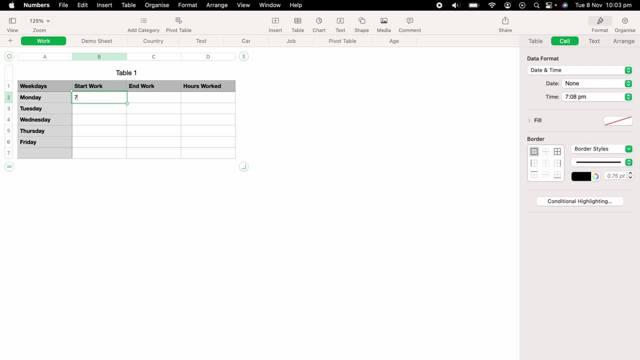 way you wish. so now let's start entering the work times. let's say this person works at seven in the morning, we'll enter seven colon zero zero, and this will indicate that this person has started work at seven am. and let's say this person finished work at five pm. so we'd put 17 colon zero zero. 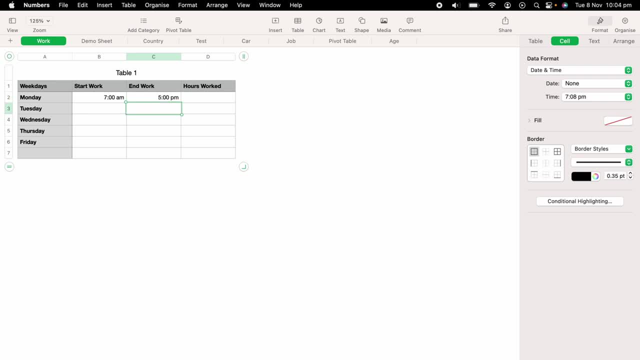 and this will indicate that this person has finished work at five pm. now just clicking a five will not work. as you can see, this does not indicate a time. however, if you don't want to use a 24 hour clock, you can do it manually by pressing five, colon, zero, zero space and then pm, and this will work as a time you have to make. 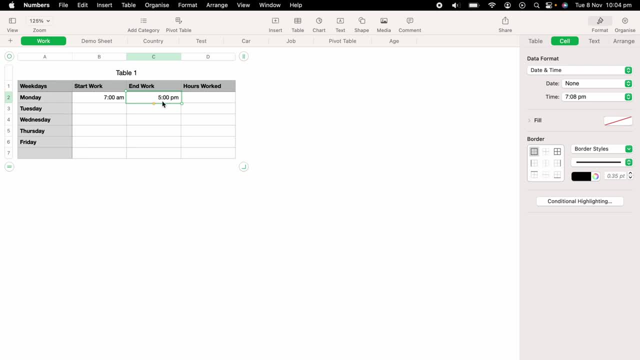 sure that you type in the times correctly. i'll just skip this part and i'll quickly fill in all the times. so now, with all the times in, let's work out how many hours this person has worked. so let's click into d2 here and we want to press the equals key on the keyboard. you first want to select the. 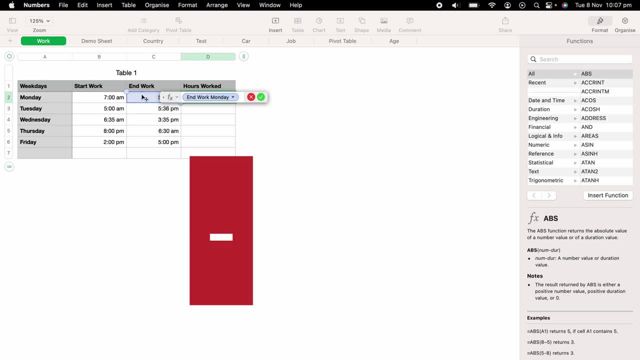 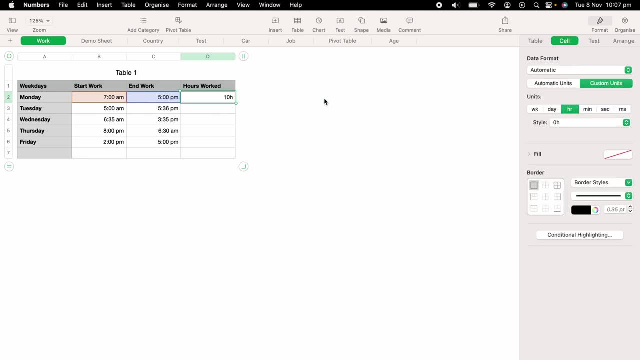 end of the working day. here in c2 then you want to press the minus key and select the start time. in b2 then you can press the enter key or this little green tick and there as you can see the hours worked. at 10 hours you can change the style on the right hand side here. 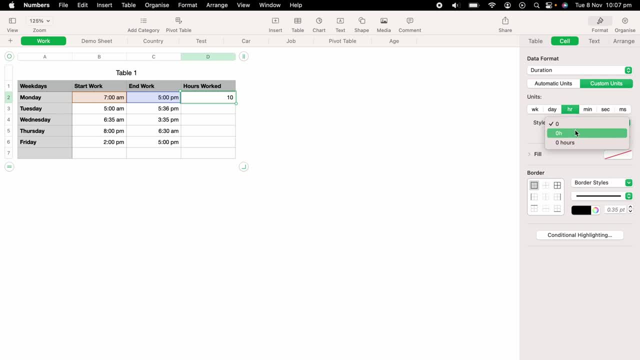 and you can select all the different ways, how you want to display the times. now, with d2 highlighted what you can do, you'd see this little yellow tab here. you want to click it and hold and drag into the rest of the cells below. as you can see here on thursday: 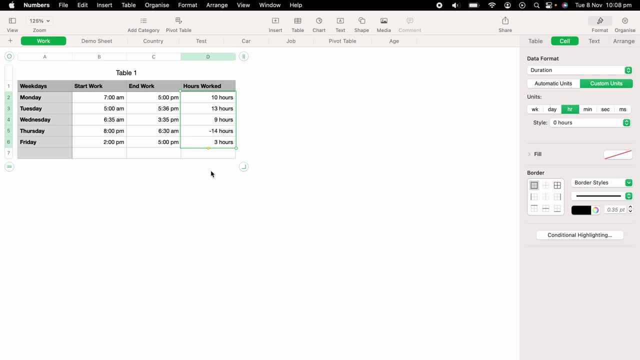 it's indicating this person has worked minus 14 hours. as this person has worked a night shift and is unable to work it out. however, we'll show you how to do that now. so let's press the equals key to bring up the function box and we need to use the if function, so we'll type if, then open bracket. 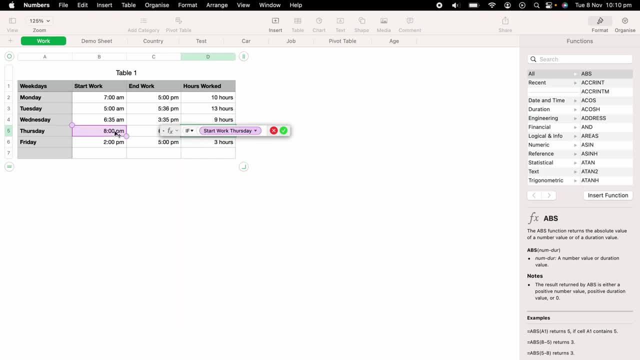 then you want to select the start of the working day in b5 and it's greater than the end time hyphen- end time again. now you want to type in a plus one hyphen- end time again, close bracket minus the start time- and you want to press the little screen, tick or enter. as you can see it's. 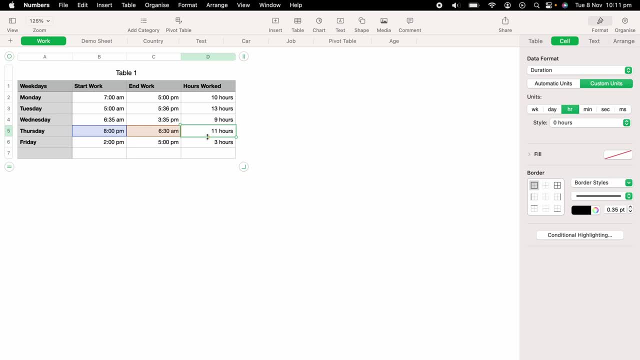 now worked out that this person has worked 11 hours. what you want to do is you want to drag this up into the other cells and down into the bottom cells. nothing actually changes, however, if these are changed to night shift hours. it will quickly work out for you. let's change this bottom.